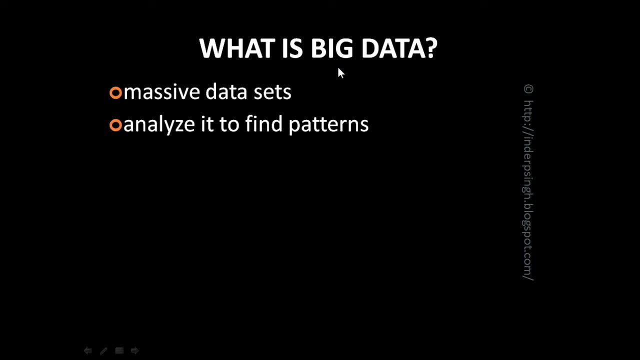 data interview questions and answers in between. Now, big data is a term used to refer massive data sets that you can analyze to find patterns. Big data needs methods to extract insights from data. Such data sets can be too big or too complex, or too varied or too dynamic to be processed by. 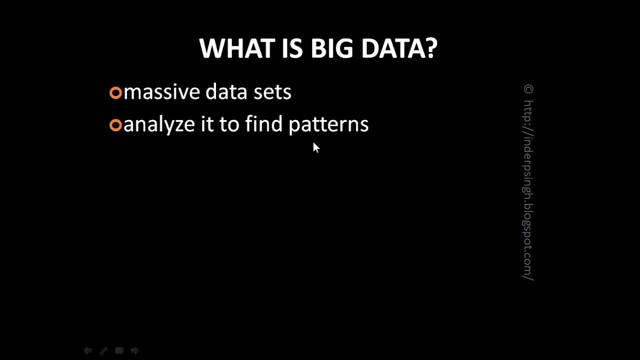 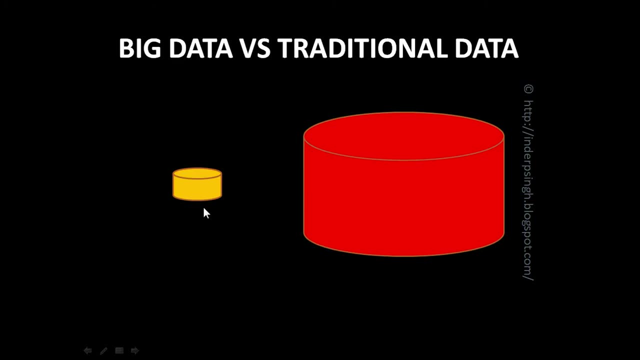 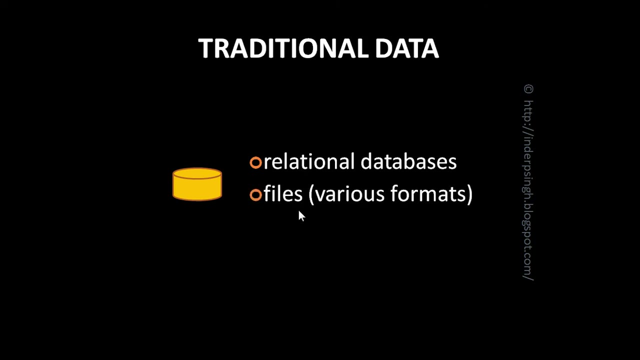 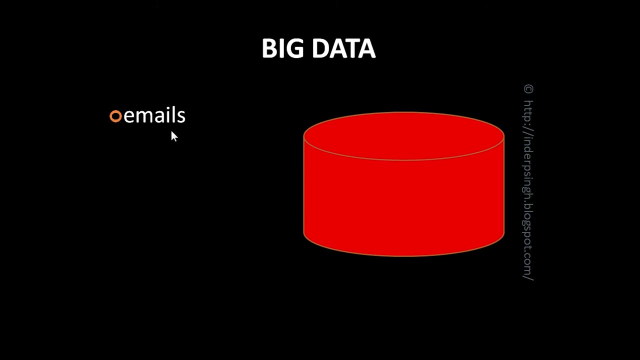 traditional database management systems and their related software applications and procedures. Now this is big data versus traditional data. Traditional data comes from relational databases and files in various formats. Big data comes from multiple sources, including emails, messages, devices like mobile devices, cameras, RFID readers and. 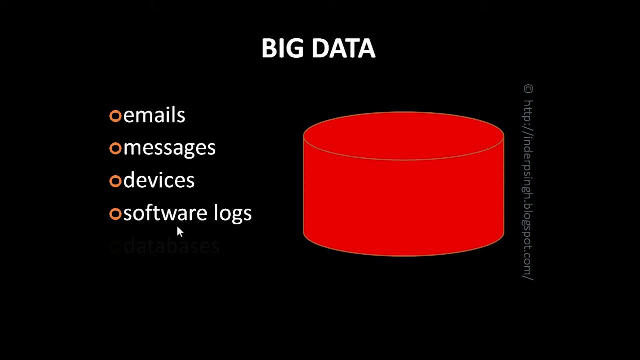 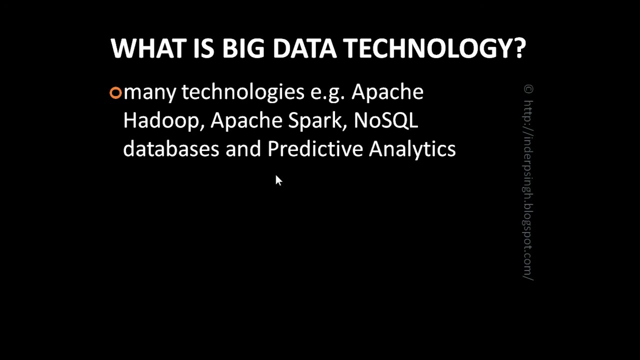 wireless sensors, software logs and databases. Big data synonyms can be large data, massive data, big data, digital data and many more. be large data, massive data, lots of data or large data volumes. Next, what is big data technology? There are many big data technologies like Apache, Hadoop, Apache. 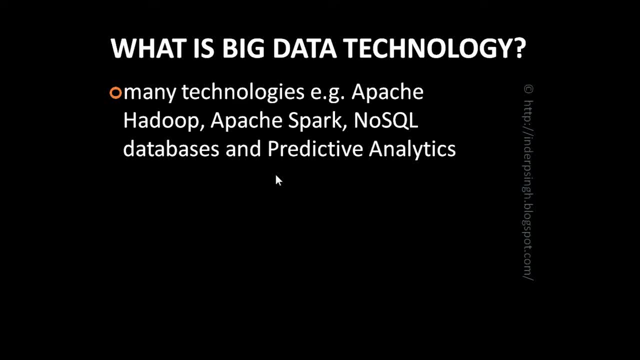 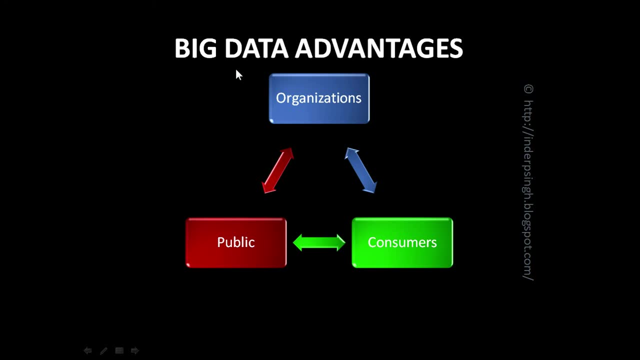 Spark, NoSQL databases and predictive analytics. Big data technologies allow organizations to analyze their operations and take informed decisions faster. Next, let us see the big data advantages. The advantages of big data for organizations are that they can get new customers retain their existing. 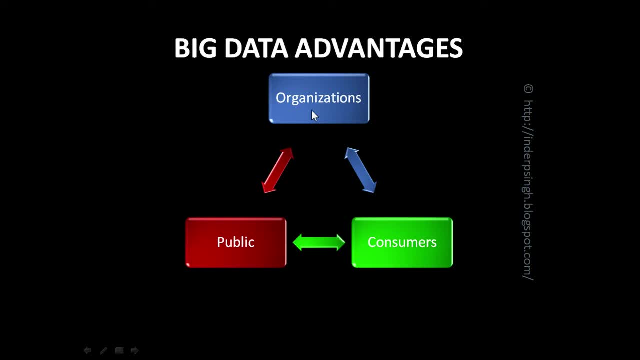 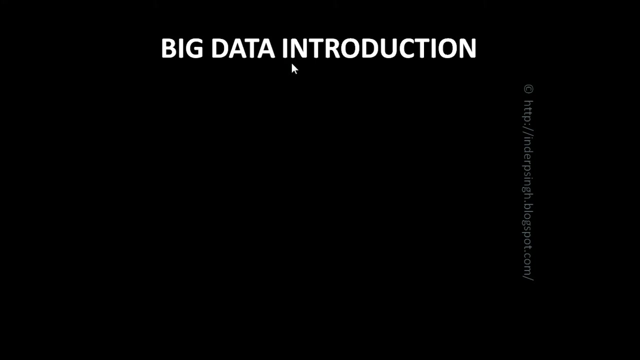 customers, increase revenues and decrease costs. The advantages of big data for consumers are personalized service and more features based on existing data. The advantages of big data for the public are health benefits and social benefits. Next, let us see big data introduction. Each one of us are creating and using big data daily. For example, if you search, 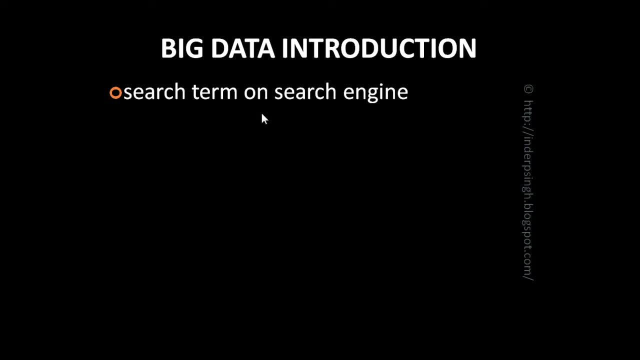 a term on a search engine like Google. the search engine uses big data to provide search results. If you search a product on an e-commerce website like Amazon, you see recommended products. The recommended products are the products that are available on Amazon. The 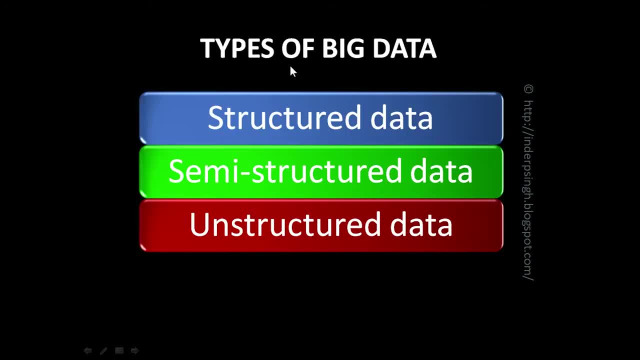 recommended products are the products that are available on Amazon. The recommendation engines use big data. Let us continue to understand what is big data concept and big data meaning. Now, types of big data are structured data, semi-structured data and unstructured data. Structured data is data that is. 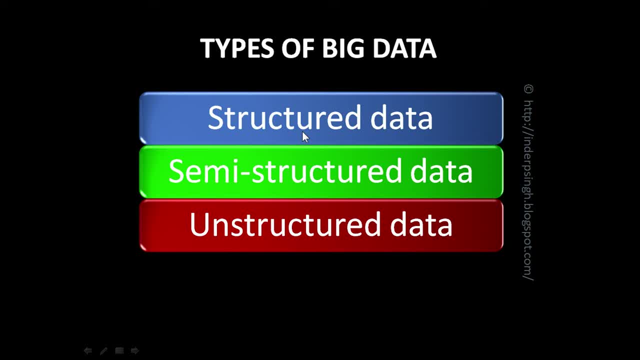 organized, labeled and can only exist in a fixed arrangement. Structured data examples are the tabular data that we see in spreadsheets and relational databases. The recommendation engines use big data to provide search results. The Semi-structured data is data that may be organized but does not follow a fixed arrangement. 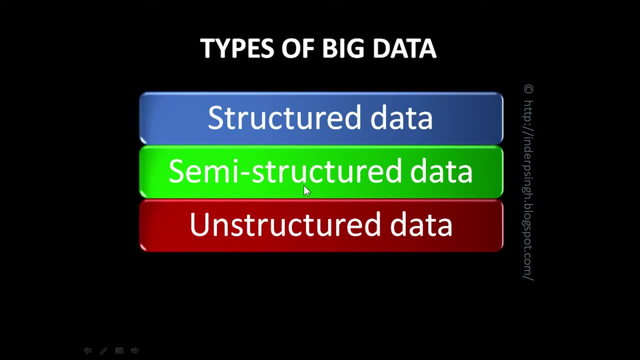 Semi-structured data. examples are data files in XML and JSON formats. Unstructured data forms a majority of big data. Unstructured data is data that is neither organized nor follows any fixed arrangement. Unstructured data examples are text files, images, audio files, video files, emails and social media data like tweets and blog posts. 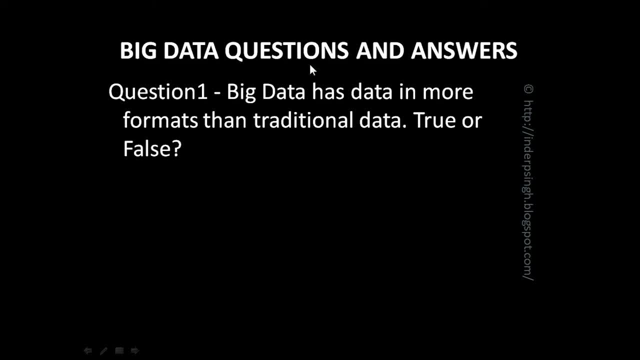 Now let us see some big data interview questions and answers. Question 1. Big data has data in more formats than traditional data. True or false? The answer is true. Next, how does big data benefit a company? Increase revenues, decrease costs, acquire new customers, or all of the above? 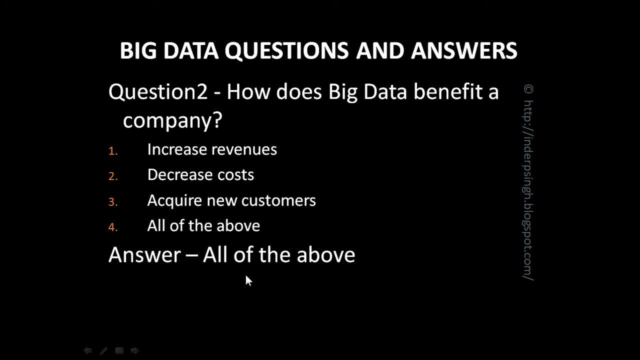 The answer is all of the above. Next question 3.. Which type of big data is most like traditional data, Whether it is structured data, semi-structured data or unstructured data. Next question 3.. Which type of big data is most like traditional data, Whether it is structured data, semi-structured data or unstructured data. 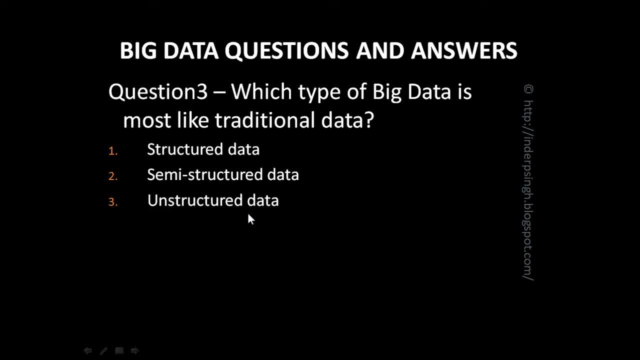 Next question 3.. Which type of big data is most like traditional data, Whether it is structured data, semi-structured data or unstructured data? It's structured data, as in spreadsheets and relational databases. Question 4. What are examples of semi-structured big data? 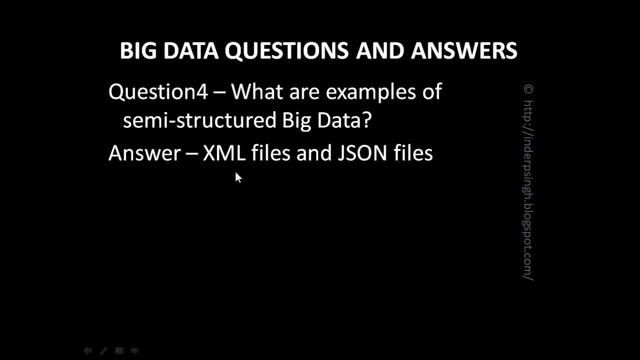 The answer is XML files or JSON files. What is big data definition? Actually, there is no single definition of big data. Also, the term big data is evolving over time. But you can form your own definition of big data when you learn about the characteristics of big data. 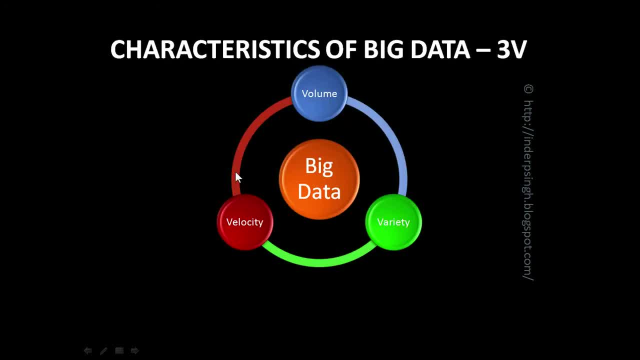 So let us see big data characteristics now. There used to be big data 3V. These were volume, variety and velocity. Then came 4Vs of big data With the addition of veracity. Now there are 5Vs of big data. 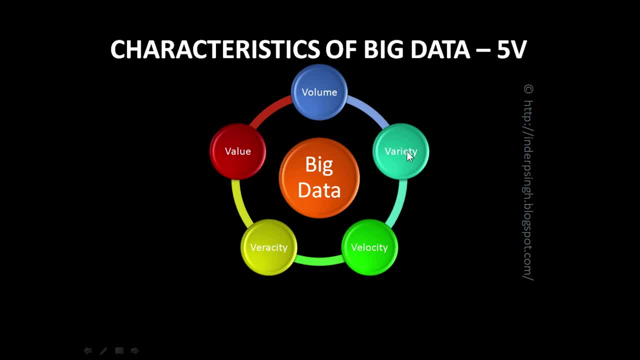 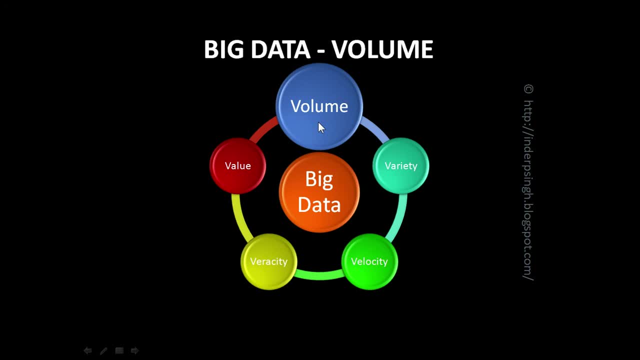 The 5Vs of big data are volume, variety, velocity, veracity and value, As you can see in this big data PPT. the first V is volume. Volume is the size of data or the increase in the quantity of data. 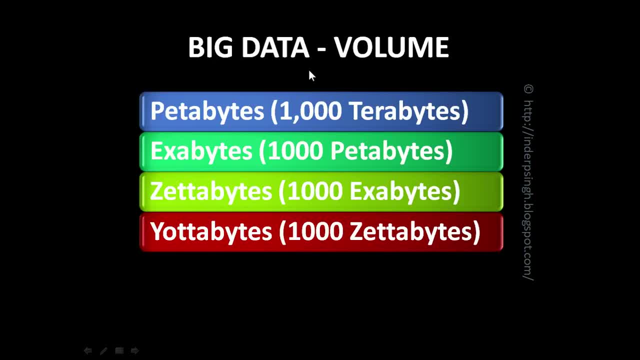 Big data is measured by its size. For example, 1 Petabyte is 1000 Terabytes, 1 Exabyte is 1000 Petabytes, 1 Zettabyte is 1000 Exabytes And 1 Yottabyte is 1000 Zettabytes. 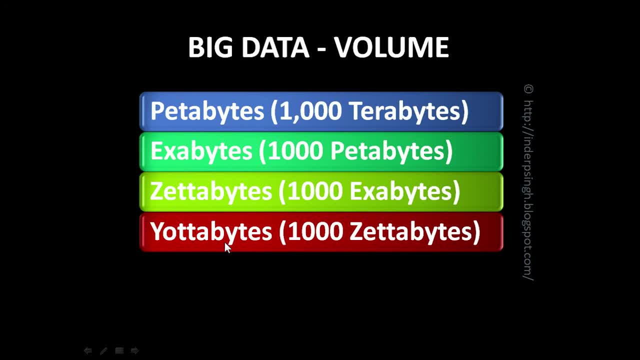 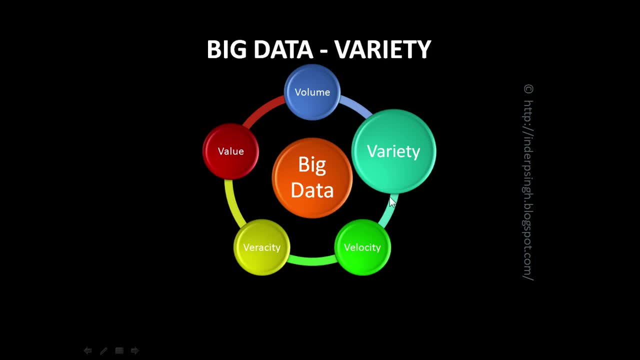 Most people in the world have a big data. Most people in the world have smart phones. These smart phones create many exabytes of data every day. Variety- The next V is variety. Variety refers to the different formats of the data. Big data can be of diverse formats. 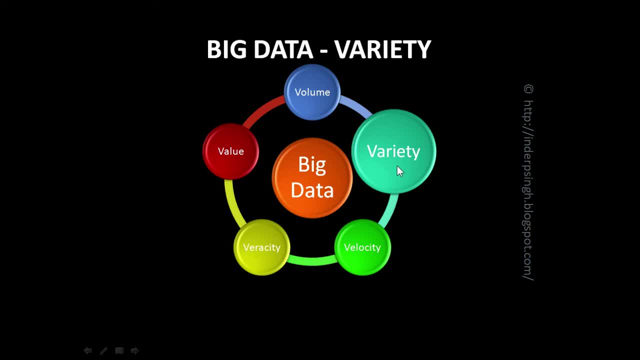 As we saw, like relational data, text, as in documents, emails and messages in social media, images, audio video and machine generated data from mobile devices, variables, sensors, RFID tags and server logs. Big data in an organization can come from internal sources, which is mostly structured data. 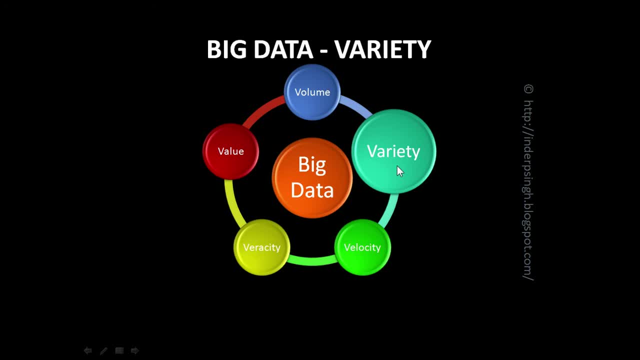 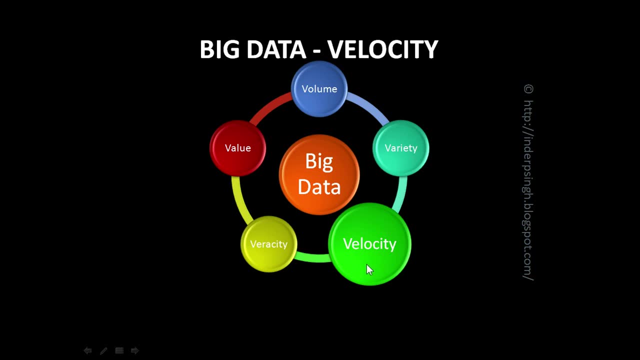 and external sources, which is mostly unstructured data Velocity. The next V is velocity. Velocity is the speed of data generation or speed of data processing. Typically, the velocity of structured data is less than the velocity of unstructured data. Big data can be processed via batch processing or real-time processing. 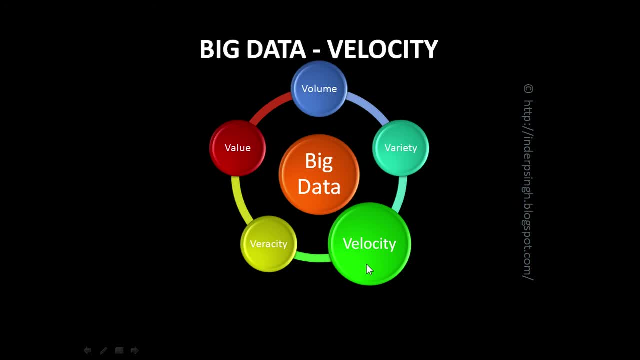 Real-time processing typically incurs more cost than batch processing. The extreme velocity of big data needs cloud-based technologies to process data quickly. By the way, velocity includes viscosity, which refers to the time difference between the transaction and the data generation. A velocity example is the hundreds of hours of video uploaded to YouTube every single minute. 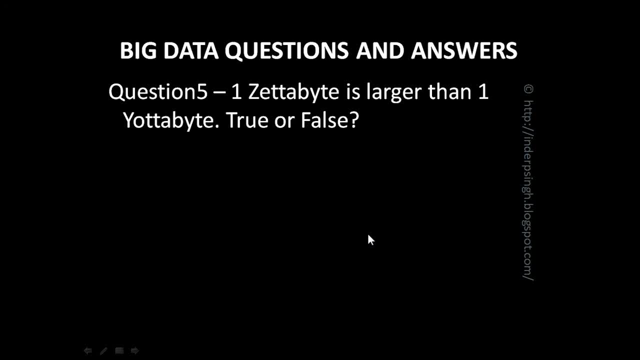 Let us see more big data questions and answers. Question 5. One zettabyte is larger than one yottabyte, True or false? Actually, it is false because 1 yottabyte is 1000 zettabytes. Question 6.: 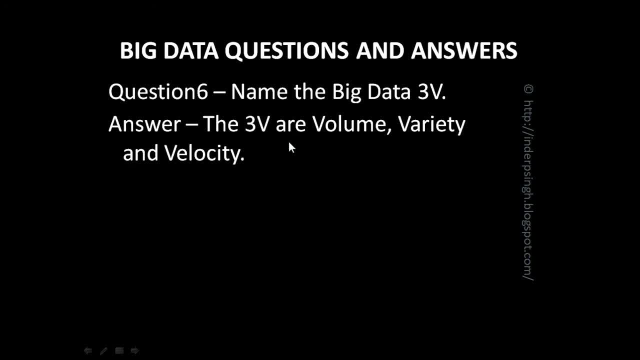 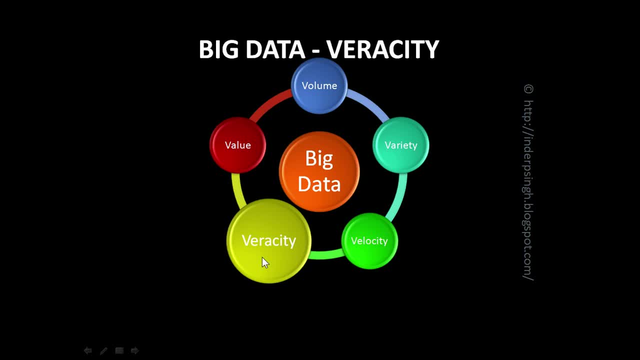 Name the big data three Vs: Veracity. the next V is veracity. veracity refers to the quality of data, meaning the accuracy, consistency and completeness of data. Big data can include data of different quality. For example, enterprise data can be of high quality. 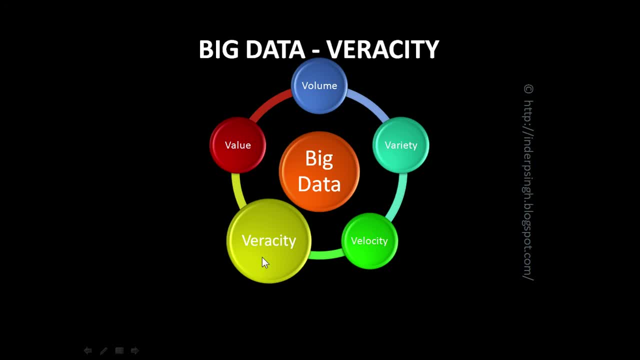 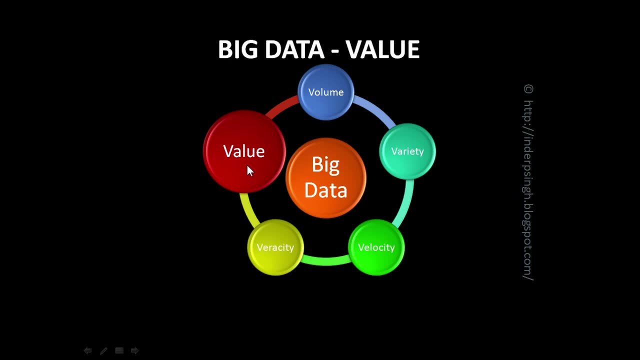 Social media data can be of medium quality and sensor data can be of low quality Value. finally, value is a characteristic of big data. Value refers to unlocking the big data into increased revenue or reduced costs or other benefits like customer satisfaction, employee satisfaction, social benefits or health benefits. 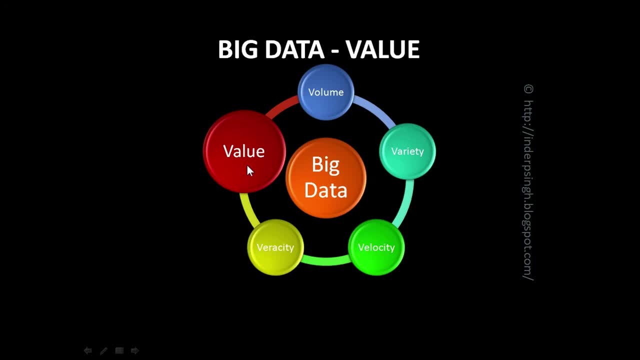 Some examples of value. in e-commerce is referring products that the customer is likely to buy. In logistics, the value example can be route optimization, leading to reduced delivery timelines and lesser transportation costs. And in utilities, value example can be reduced customer churn or customers who leave the 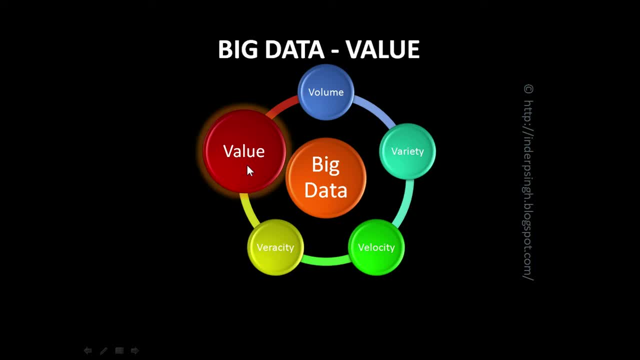 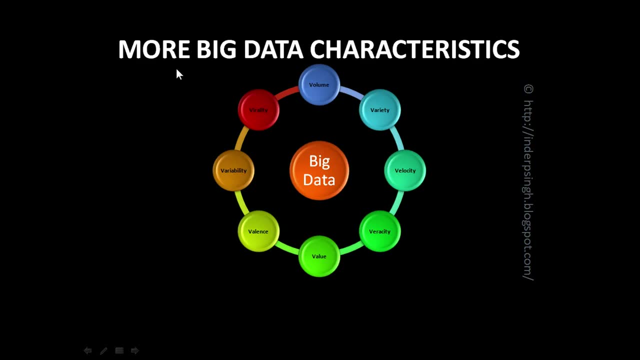 utility company Value is the most important Big data V. There are even more big data characteristics. Valence is also a V of big data. Valence refers to the connections between the data. Data with more interconnections is more complex than data with fewer interconnections. 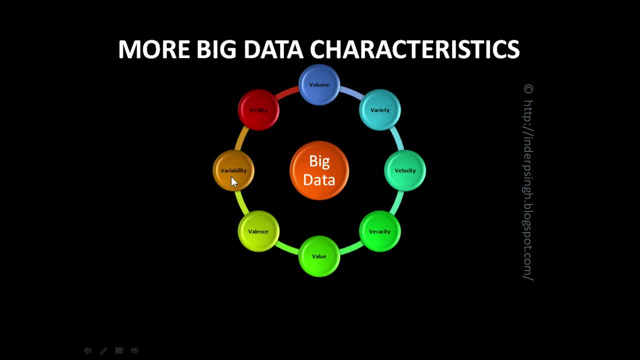 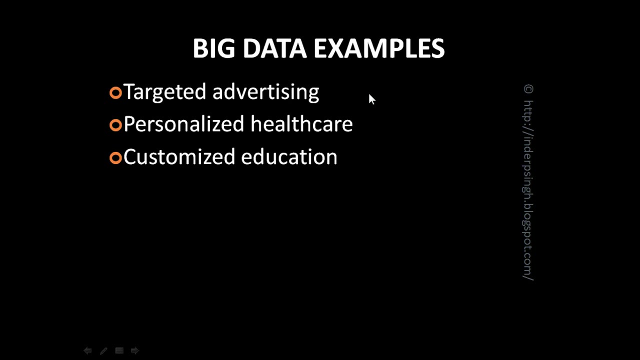 Variability refers to the data generation, consistency Meaning is the data available regularly or intermittently, And virality refers to the speed at which the data is spread. Just some big data examples include targeted advertising, personalized healthcare and customized education. Big data analytics are being used in every industry to become more responsive to customer. 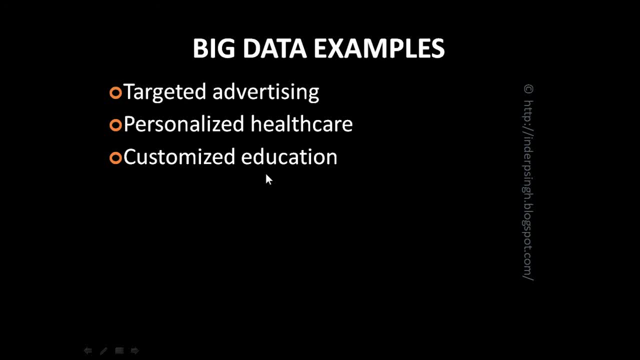 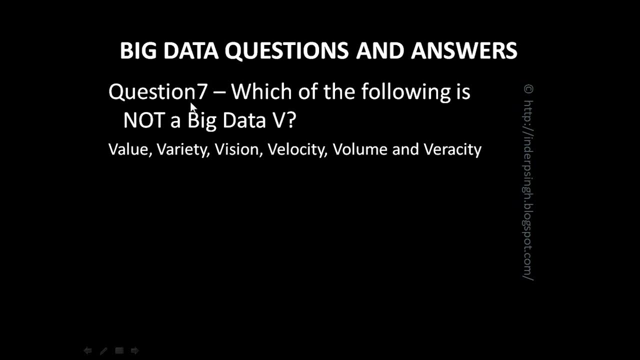 behavior much quicker. Now more questions and answers. Question 7. Which of the following is not a big data: V: Value, Variety, Vision, Velocity, Volume and Veracity. The answer is: The big data 5 Vs are Volume, Variety, Velocity, Veracity and Value. 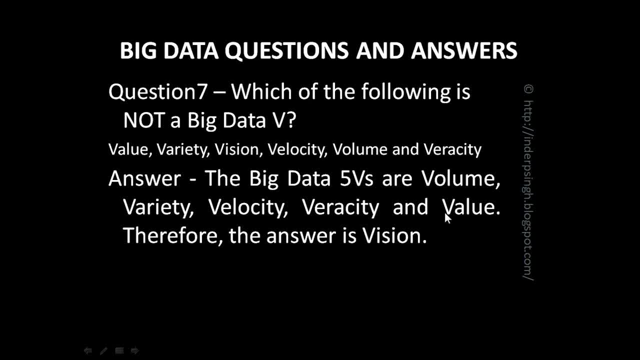 The answer is The big data: 5 Vs are Volume Variety, Velocity, Veracity and Value. The answer is The big data: 5 Vs are Volume Variety, Velocity and Value. So Vision is not a big data V. 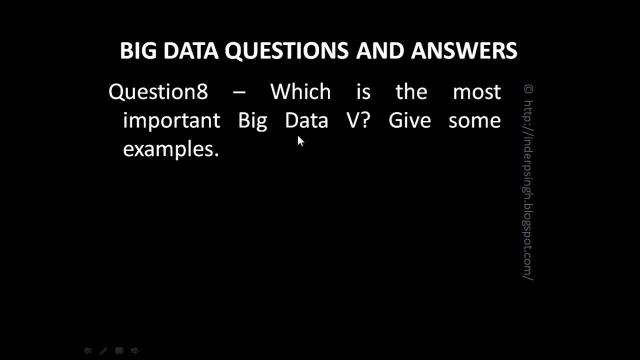 Question 8. Which is the most important big data V And give some examples. As we know, the answer is Value. Value is the most important big data V. Some examples are recommendation in e-commerce, route optimization in logistics and customer upselling. 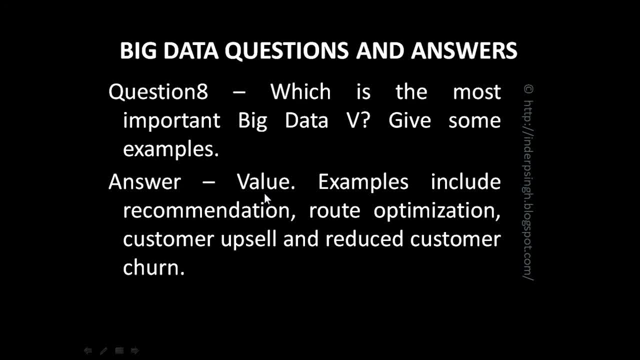 And Reduced Customer Turnover in Utilities.